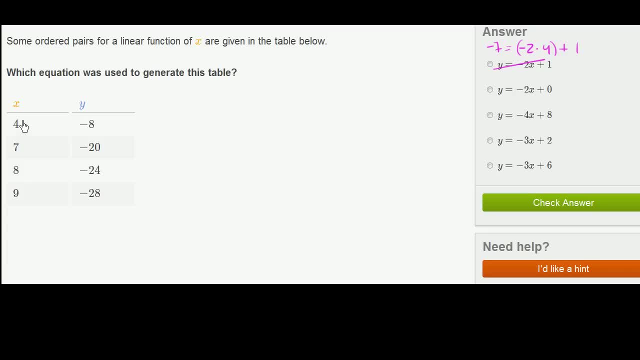 right over here, So we could just rule it out. Whatever equation should have been able to generate for any given x, for any of these x's, should generate this y right over here. Now let's go to this next equation: y is equal to negative 2x plus 0.. 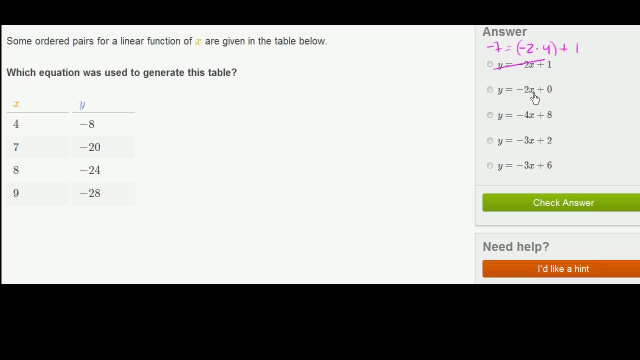 So when x is 4, y would be negative 2 times 4, which is negative 8.. So this second equation seems to be capable of generating this first set of points: When x is 4, y is negative 8.. 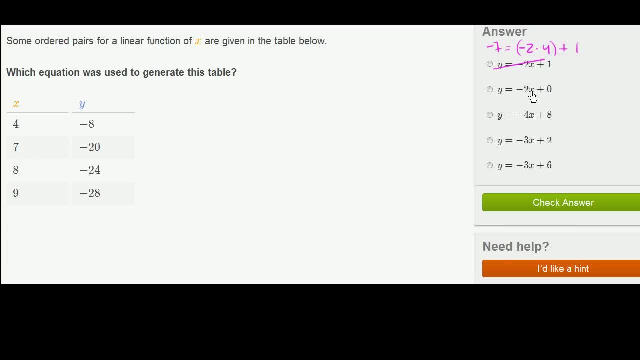 But let's see if it works for the second one right over here. When x is 7, you would have negative 2 times 7. Right, Which is negative 14. But here, when x is 7, y is negative 20. 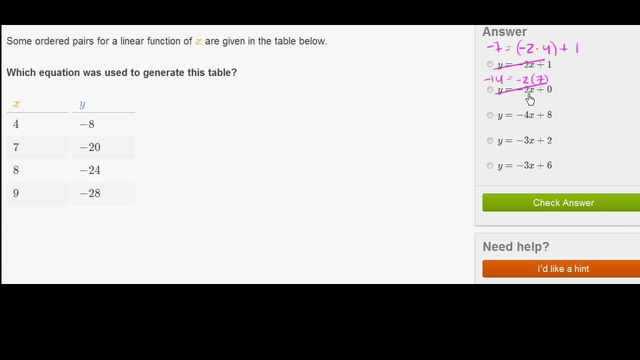 So this one we can rule out, because when x is 7, y does not equal negative 20, like this point right over here. So we'll rule that second one out. Now let's look at this third one. y is equal to negative 4x plus 8.. 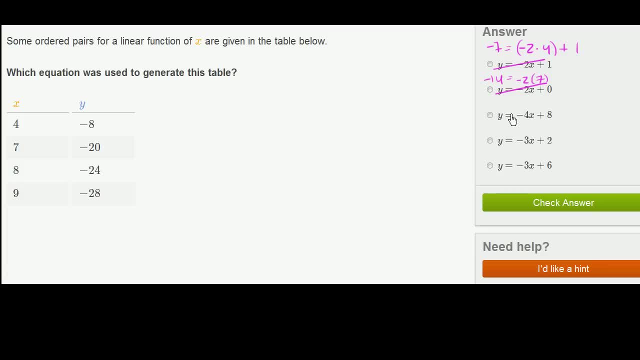 Well, we could go to this first point again. When x is 4, let's think about what happens when x is 4.. So when x is 4, you have negative 4 times 4., Which is negative 16 plus 8,, which is negative 8.. 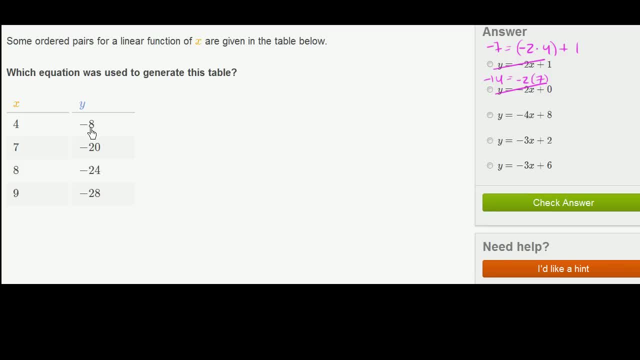 So it seems to be able to generate this first point When x is 4, y is negative 8 for this equation right over here. Now let's see what happens when x is 7.. So negative 4 times 7 is negative 28.. 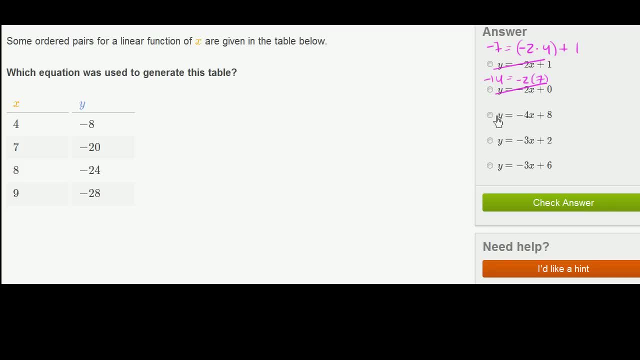 Negative. 28 plus 8 is negative 20.. So this candidate is starting to look pretty good. It's pretty good, It satisfies these two points And, frankly, for any of these linear functions, if it satisfies any of these two points. 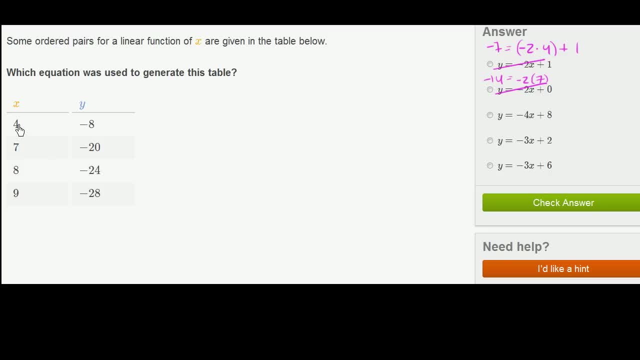 if some linear function generated all of these, if some function can generate any two of them, it will satisfy all of these, Because two points define a line, But we can verify it right over here. So let's see what happens when x equals 8..